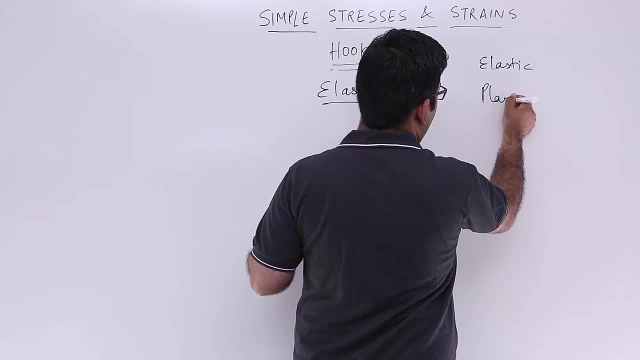 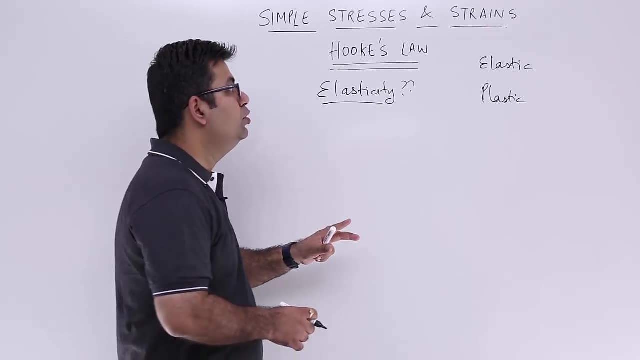 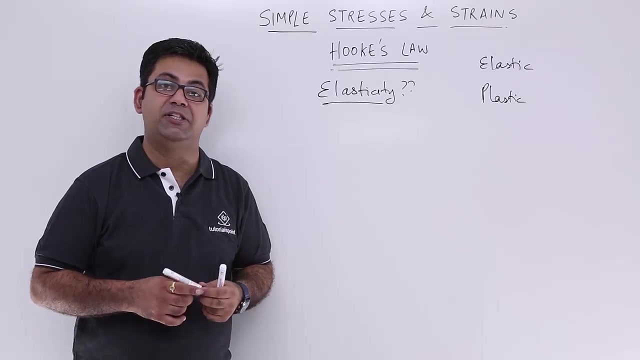 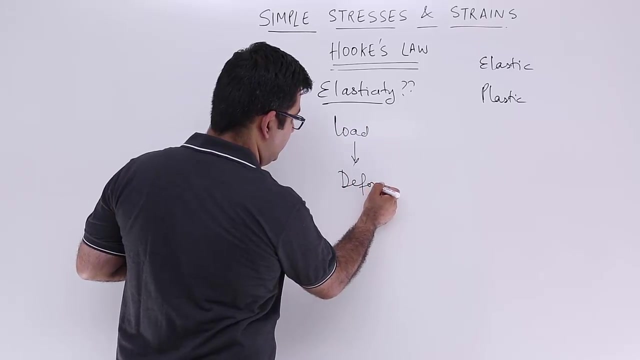 The first deformation was elastic and the other deformation was plastic. Okay, so elasticity has something to do with both of them. So when you put load onto a body, it gets deformed, Alright. so you put load, load brings about deformation, Alright. now this deformation? 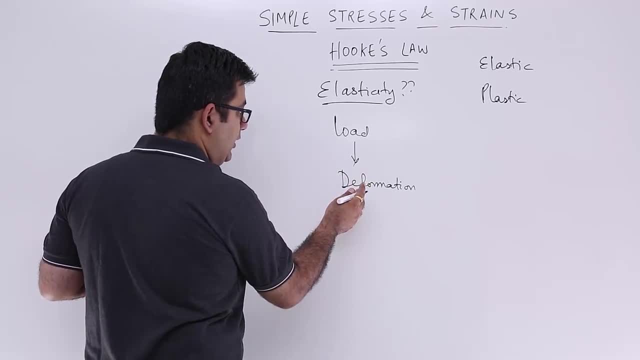 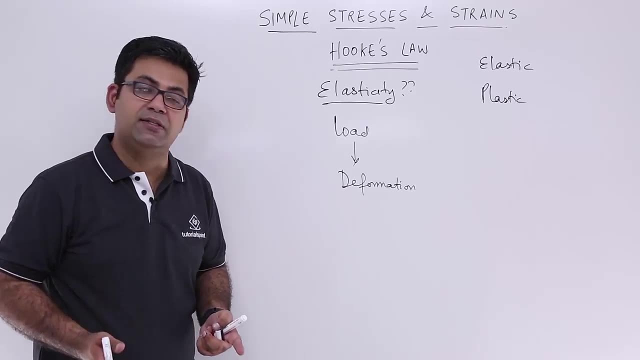 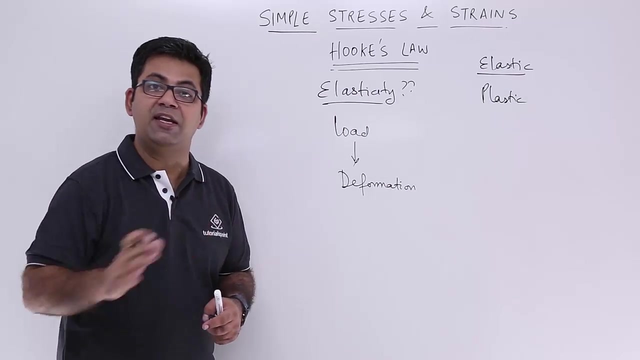 is elastic. Okay, if you, let us say, remove the load. if you remove the load, the deformation vanishes. So if such a phenomena occurs, then your deformation that occurred was elastic. Okay, so the deformation vanishes, or the material or the body goes back to the original shape. 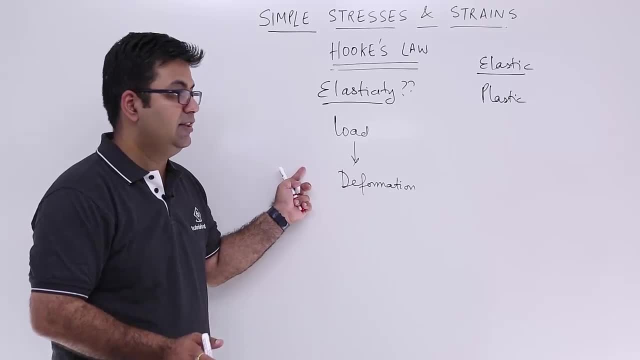 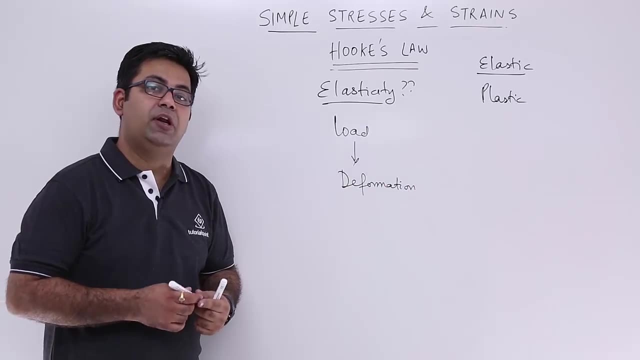 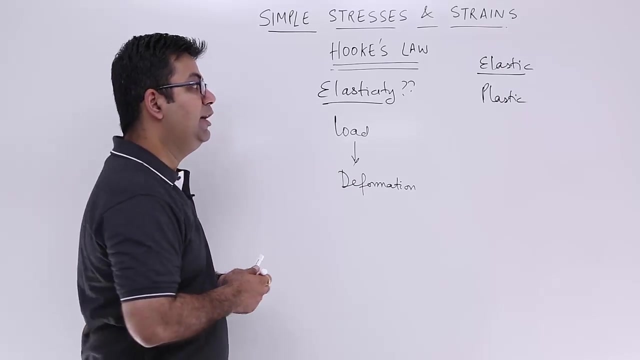 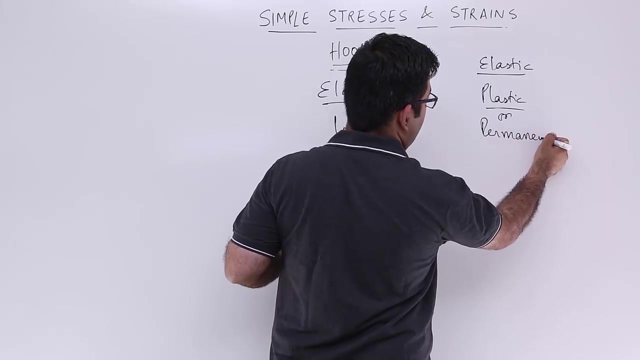 that was earlier, before the loading began, then that kind of deformation is called elastic. Okay, but if, even after removal of the load, the body is unable to trace back to its original shape, the deformation is called plastic deformation or it has another name: permanent deformation. 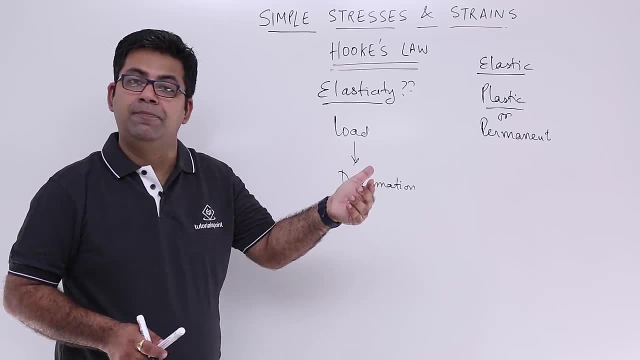 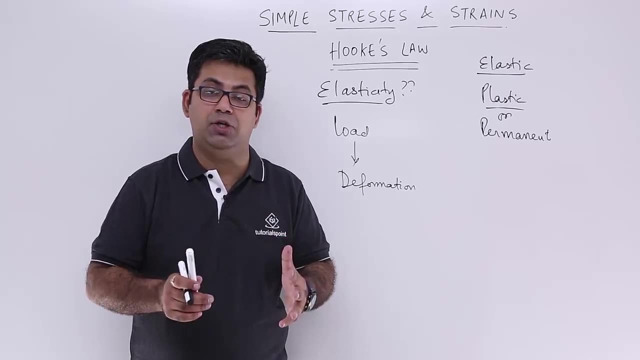 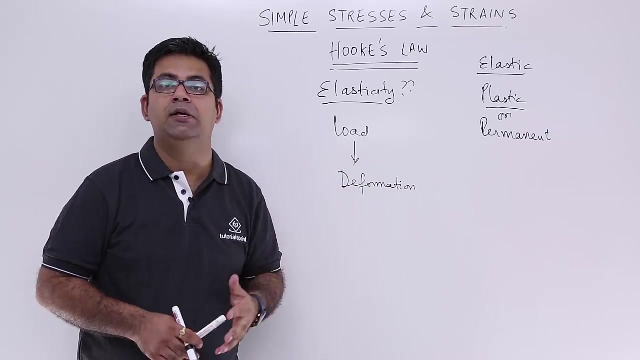 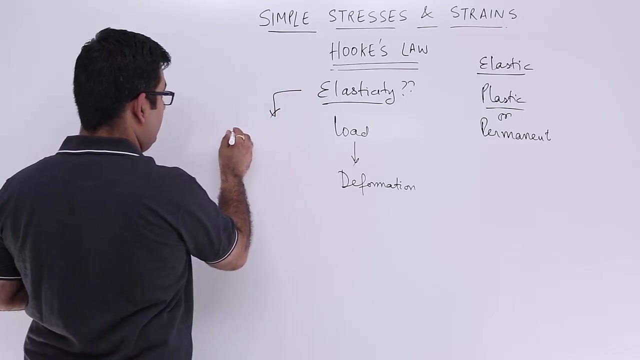 Okay, so what is this term elasticity? The term elasticity is basically the property of a material. ok, till which or due to which, upon removal of load, it traces or it regains its original shape. ok, so that is what elasticity is, that is, the property of the material. 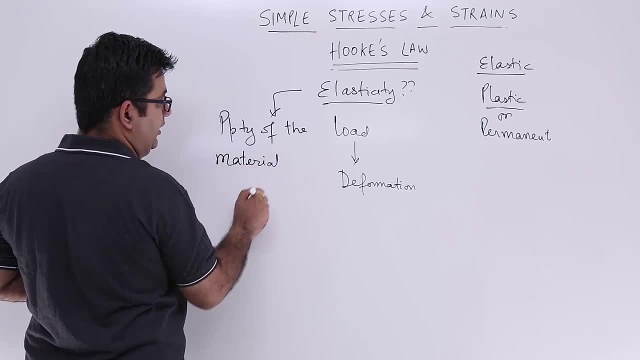 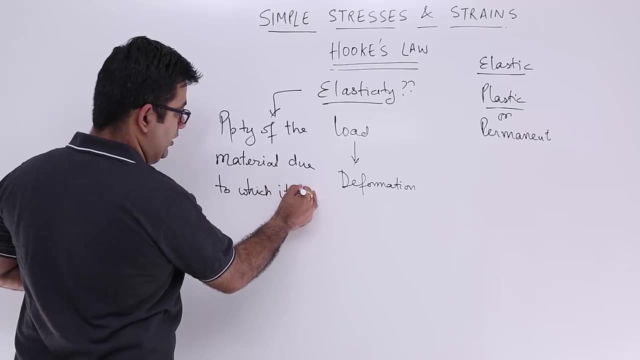 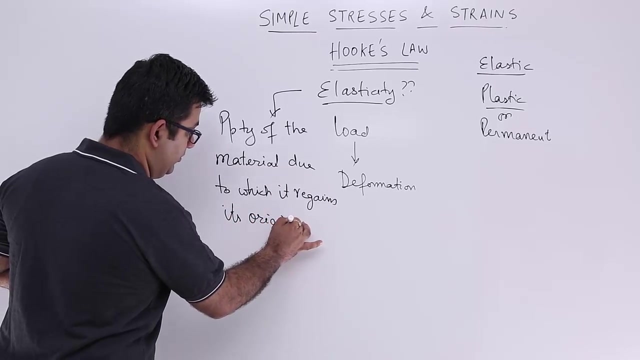 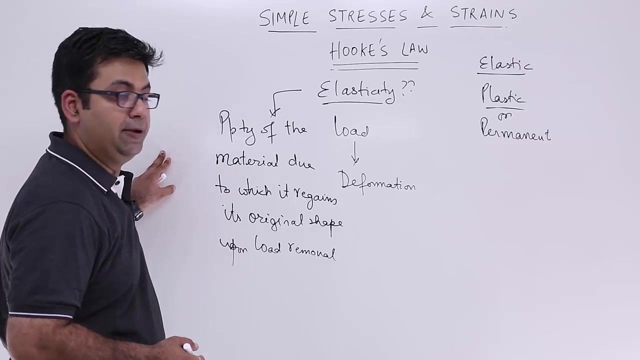 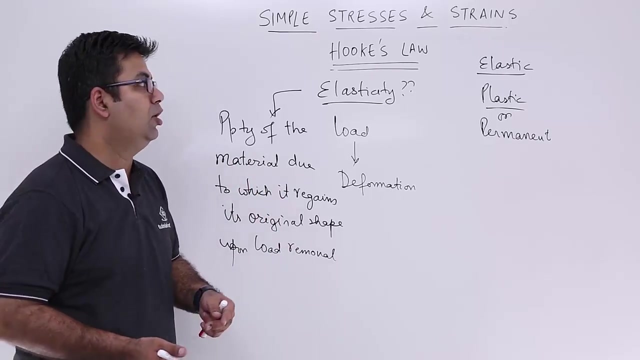 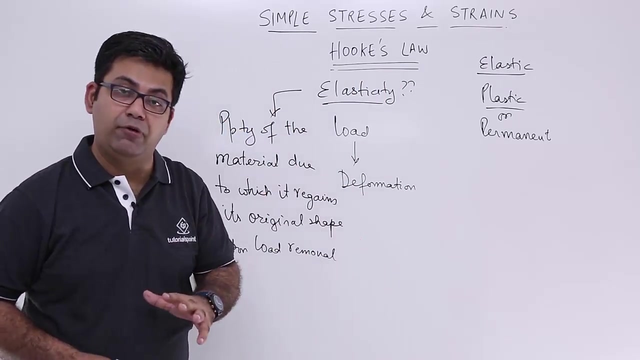 the property of the material due to which, due to which it regains its original shape upon load removal. so that is what elasticity is. that is the property of the material. that is what we call elasticity. ok, so when we start talking about this, that elastic deformation- or you can say this- is also termed as temporary deformation, or plastic deformation, or permanent deformation, and then you have a term: elasticity. 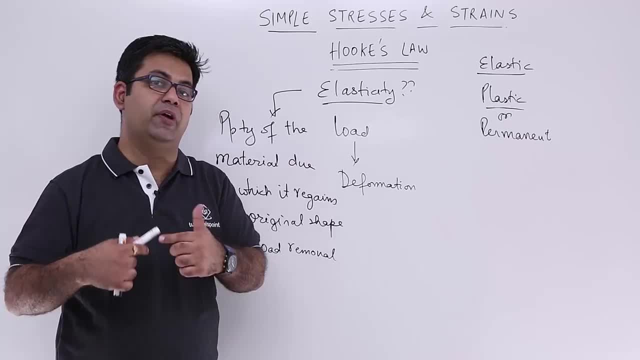 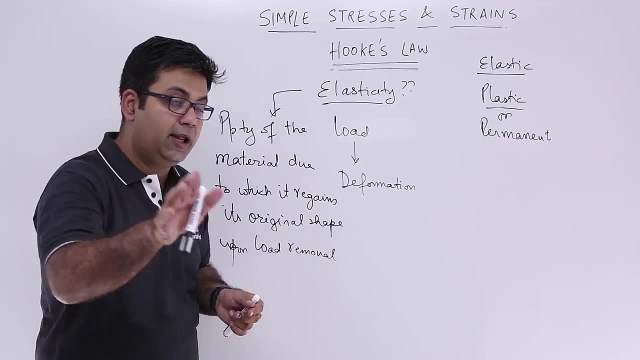 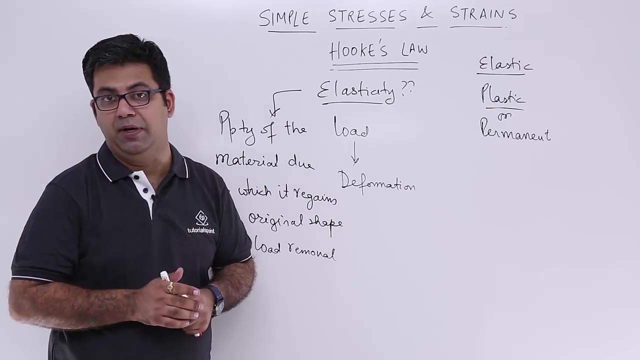 now you keep on applying load and you keep on removing it, you will witness that there is a certain value of load till which only you can get ok, ok, ok, your. you can say original shape back. you can actually regain the original shape, that point of load. if you exceed that, you cannot regain your. 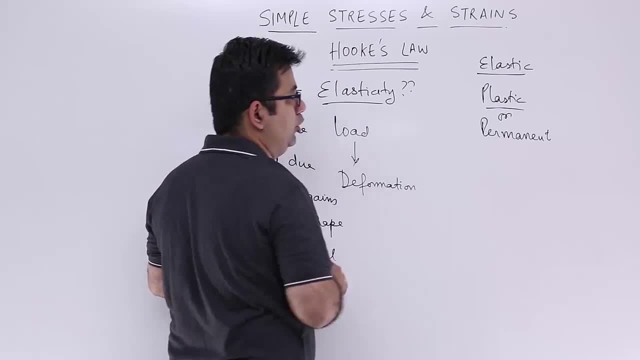 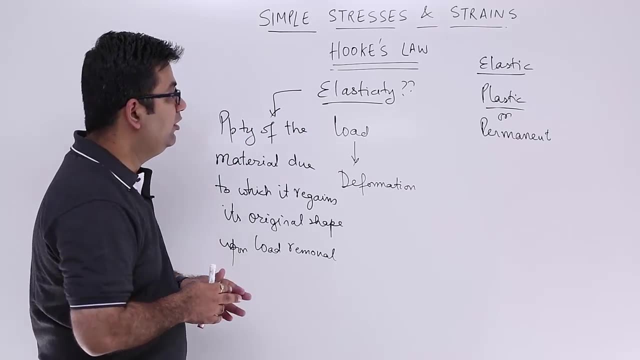 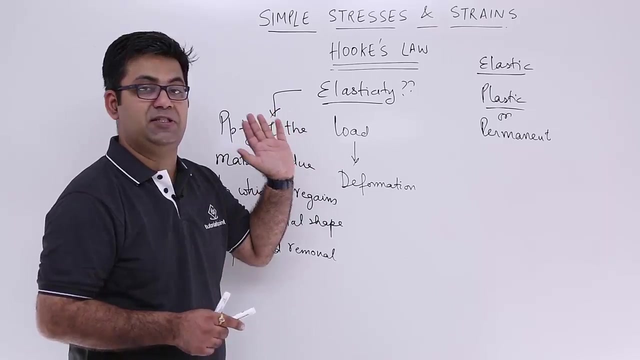 original shape. and then it is said that you have gone into the region of permanent deformation. what is that region? we will talk about that in the next video, but in this video you need to understand this: that limiting load up till which your material remains elastic. that is the original shape. can be regained after the load removal. that limit of load is called elastic limit. it is called elastic limit. so the load corresponding to this elastic limit is called the elastic limit load and the stress produced corresponding to the elastic limit is called the elastic limit stress. okay, and the strain also is called the elastic limit strain. 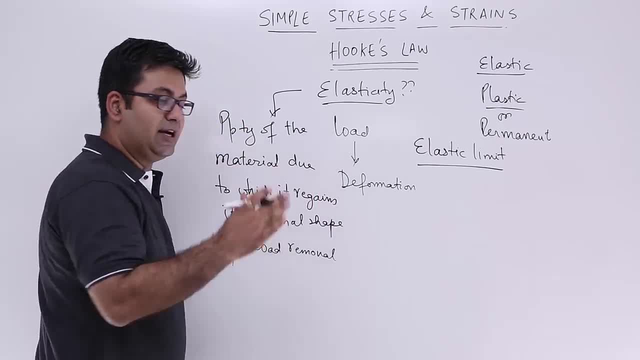 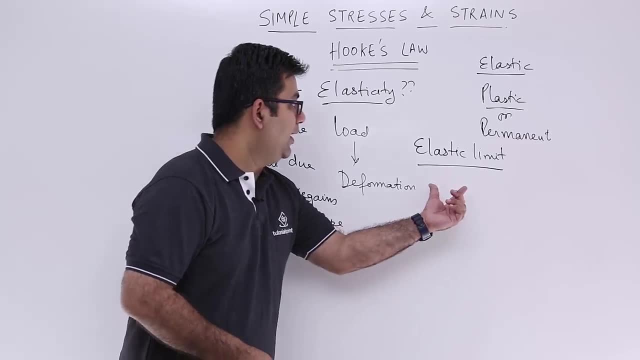 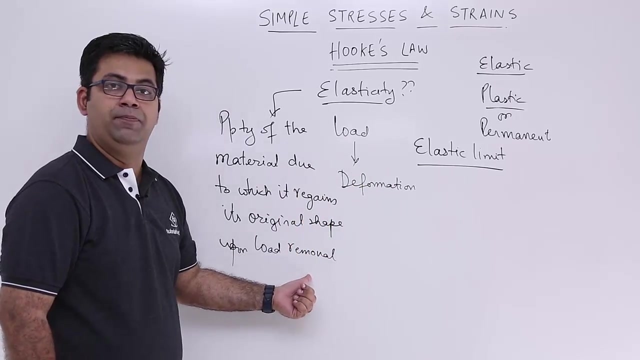 right. so in a nutshell i can say that if you load your body or if you deform your body up and until the elastic limit, you can regain the original shape upon load removal. if you exceed the elastic limit, you cannot regain the original shape. you will be under. 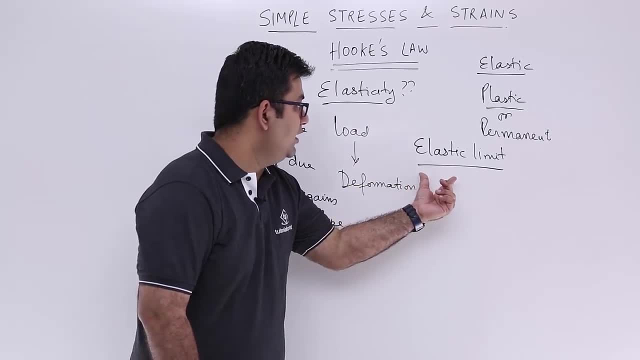 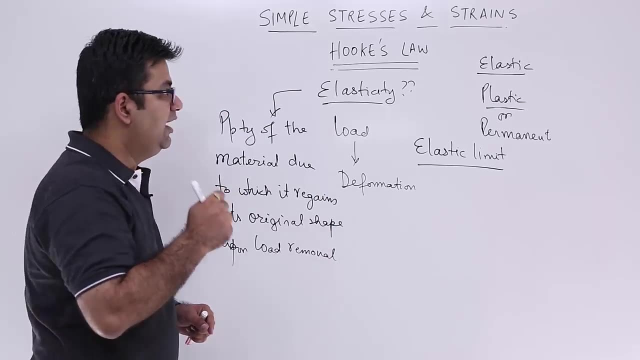 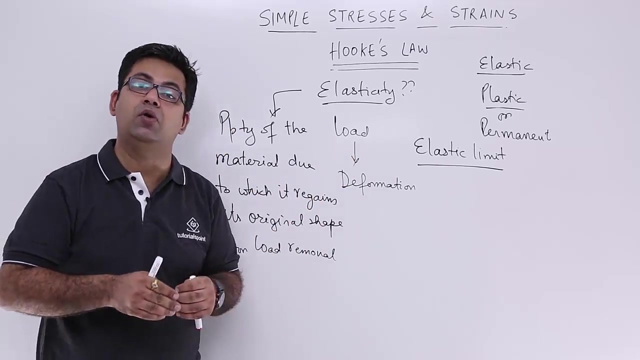 permanent deformation. okay, now this elastic limit becomes the basis of the definition of Hooke's law. so by Hooke's law we state that if your body is loaded within the elastic limit, that is, we are not going into the permanent deformation stage. if the body is loaded within the elastic 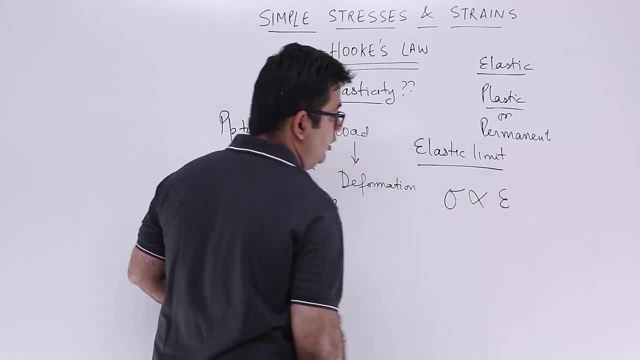 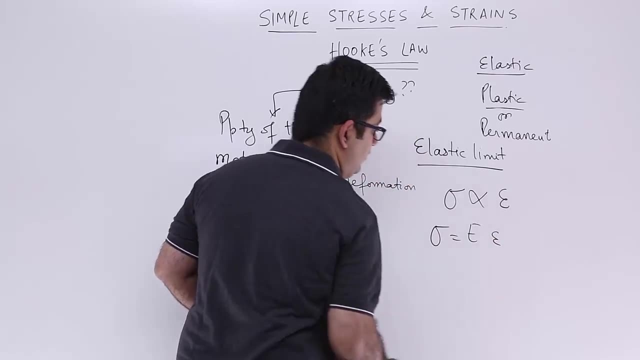 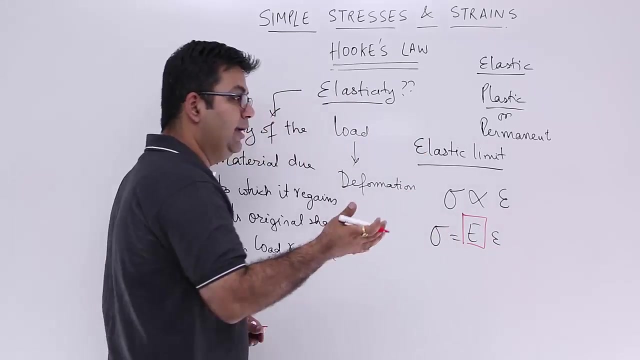 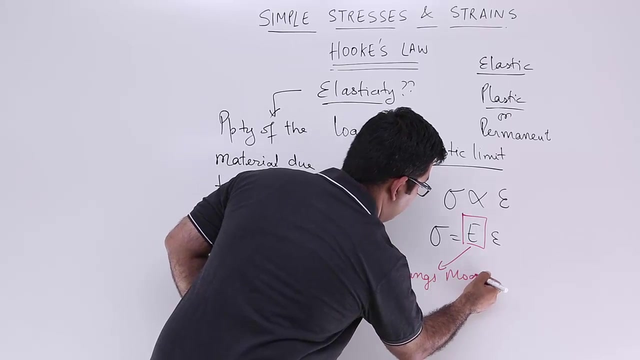 limit, then the stress produced is proportional to the strain. okay, so if you remove this proportionality sign, you will get a constant of proportionality and that is a capital E over here. this capital E is called the Young's modulus. it is called the Young's modulus or the modulus of elasticity. 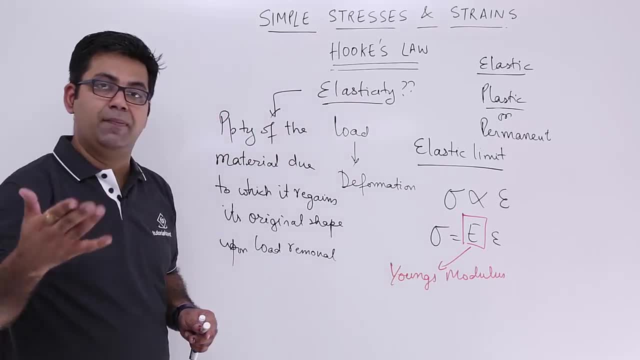 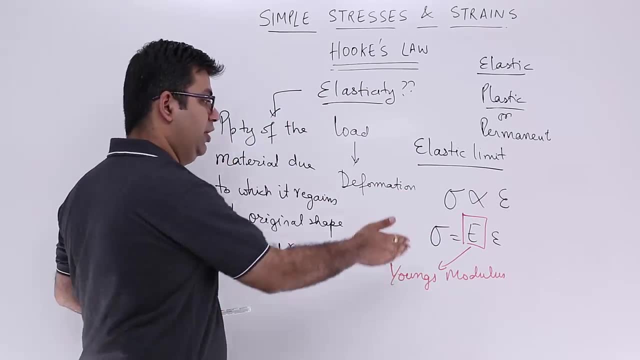 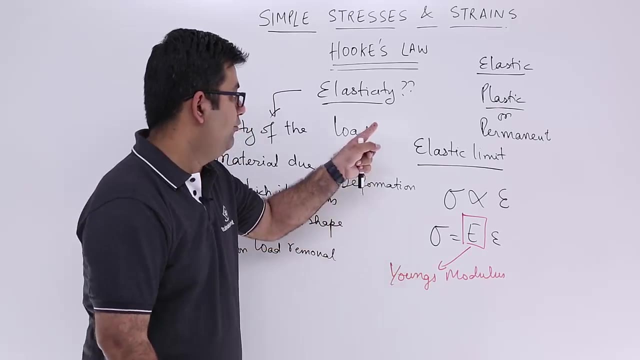 okay. so because stress has a unit of megapascal or gigapascal, strain has no stress, so the stress produced is proportional to the strain. strain has no units, so the Young's modulus will the same units as that of the stress. okay, so this was Hooke's Law, basically this equation for till the elastic limit.